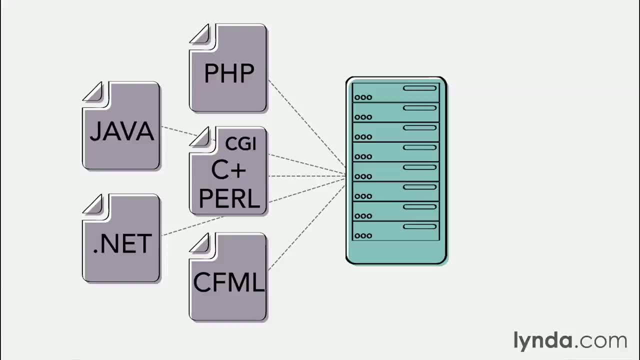 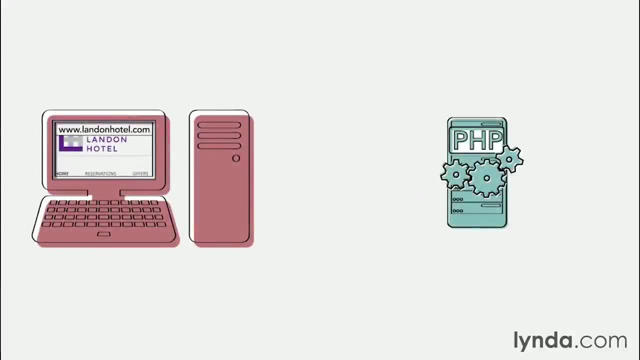 they're creating dynamic sites. Although each language is slightly different, the process for utilizing server-side scripting on a web page is pretty consistent. If a web page containing server-side scripting is requested from a server, the web server first processes the script before the page is served to the browser. Processing the script can involve pulling information from a 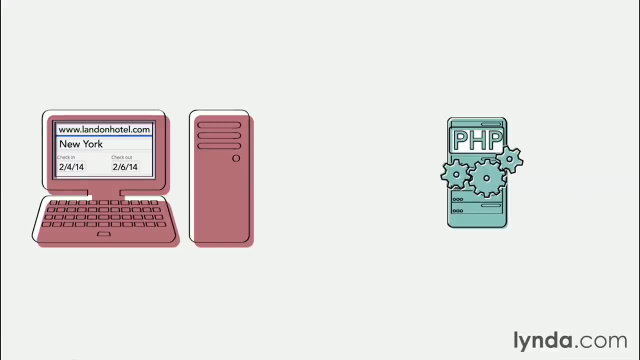 database, making a script or making a script from a browser. This can be done by using a simple calculation or choosing which pieces of content to display on the page. Once the script has been processed, the resulting content is then returned to the browser and then it's rendered. 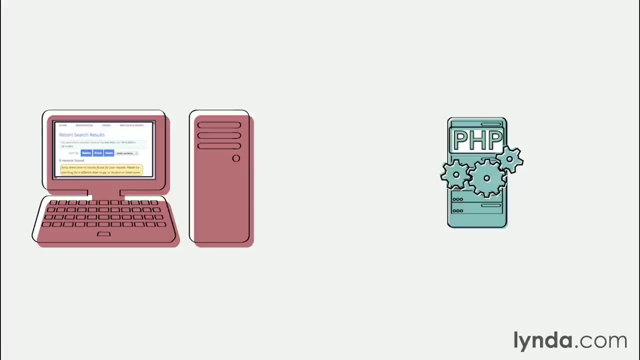 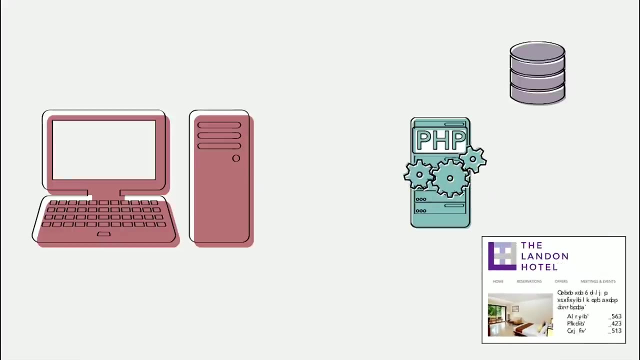 This process can occur from either a simple page request, through something like a user filling out a form, or from interacting with a specific widget. Since the scripts run on the web server prior to serving the content, the scripts themselves are hidden from the end user. This adds a layer of 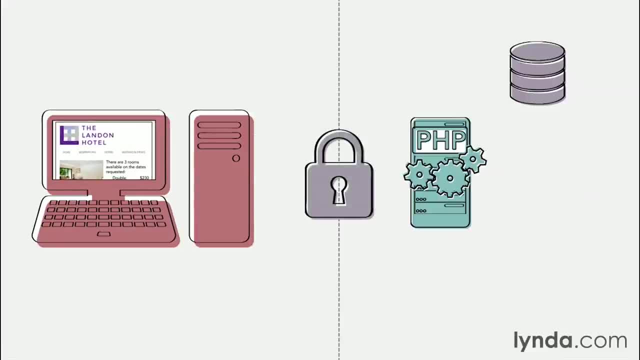 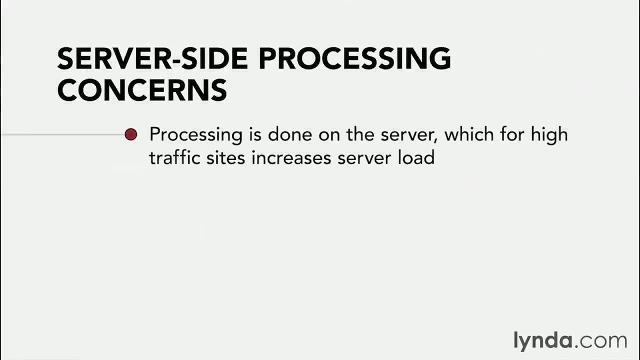 complexity to the web server. This can go beyond the website's capacity for data and code. There are, of course, some downsides to using server-side scripting. Since the processing must be done on the server, it places the burden of running the application on the web server itself. 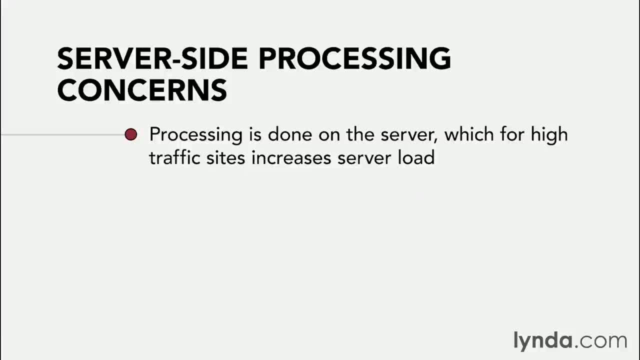 rather than the client machine For larger applications or sites with a lot of page requests. this can slow down the site or force the site to upgrade to larger or even multiple servers to handle the load. The flow of dynamic pages can be frustrating for end users as well. 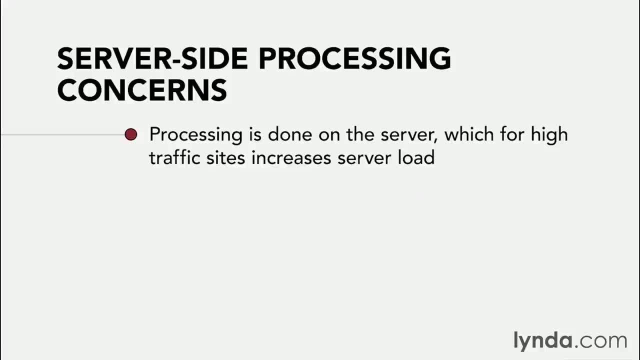 But the point is, data is actually the source of all the data in the server. It doesn't matter if the data is not doctored to the web server or if not. the data is the source of all the data in the can be frustrating for end users as well. 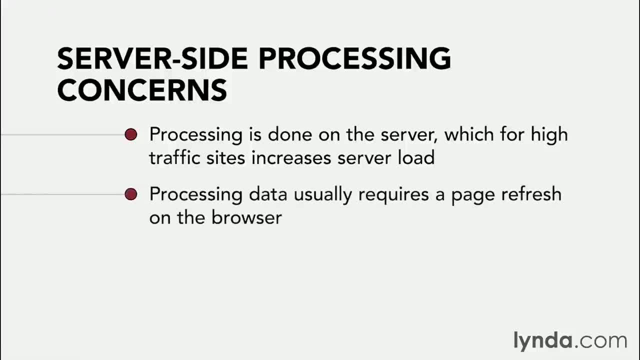 Because the server must process the scripts, there's usually a page refresh required to display new content. This is largely the reason that client-side scripting has gained in popularity, as well as the development of techniques that run server-side scripts without requiring page refreshes. 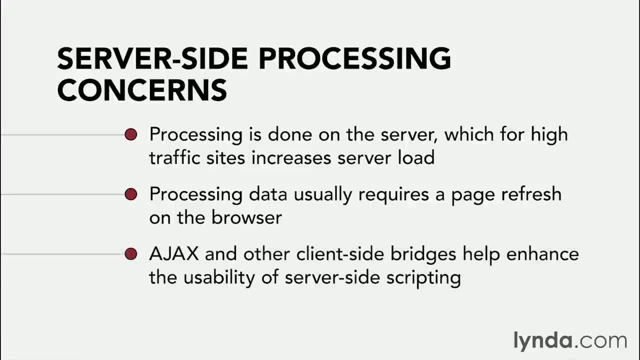 To be honest, the terms client-side scripting and server-side scripting are becoming rather nebulous. Developers have become very adept at using JavaScript to blend the two methods together into a seamless user experience. If web development interests, you be sure you focus on not just the server-side software. 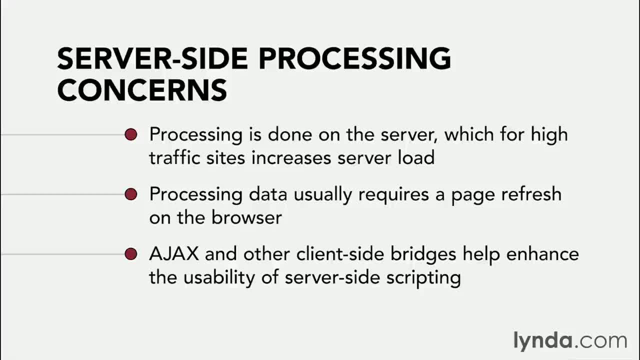 that we're going to be exploring in this chapter, but also how JavaScript is being increasingly used for more powerful client-side scripting and as a method of controlling scripting on the server as well.